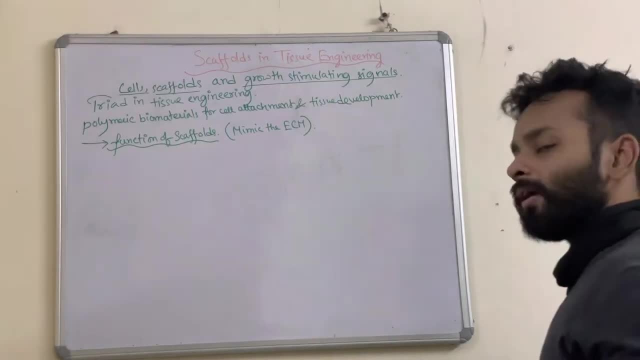 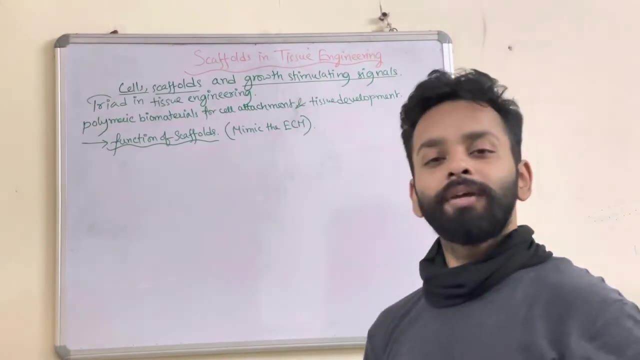 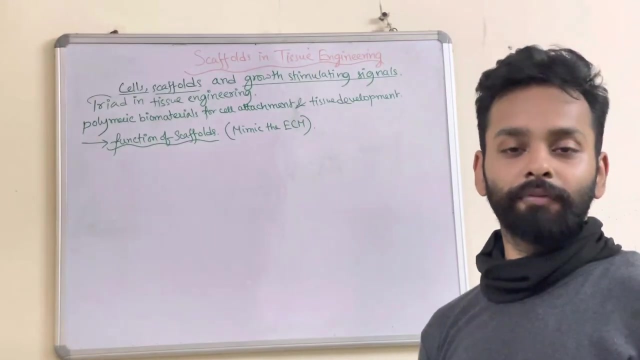 Hello and welcome to another video in the lecture series entitled Advanced Biomaterials. So in today's lecture we will look at a very important aspect of tissue engineering, very important construct which is used in tissue engineering, which is known as scaffold. So we will 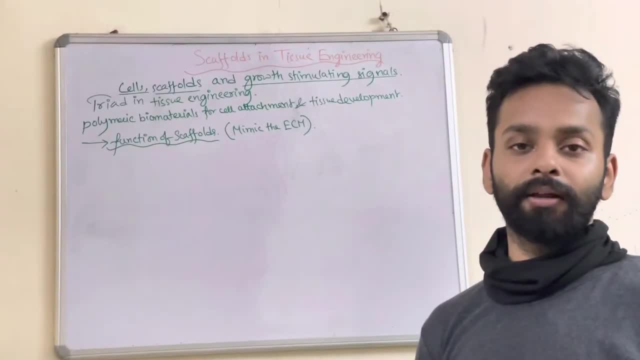 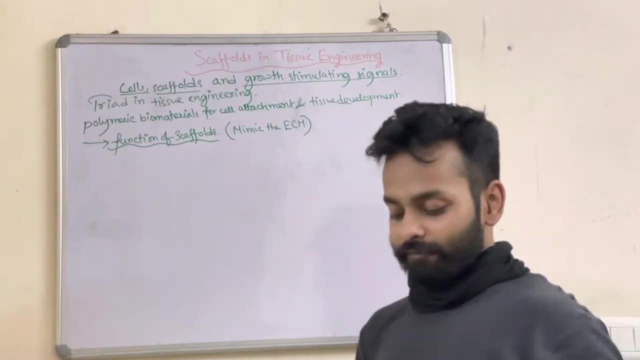 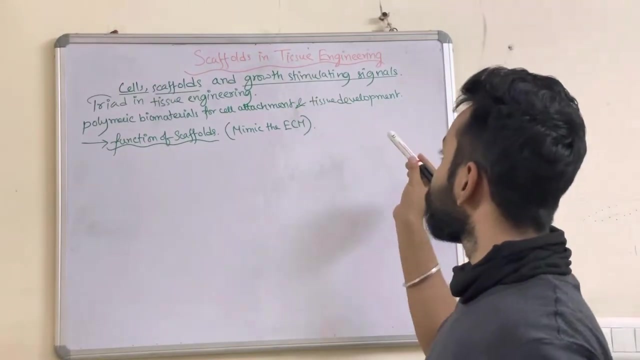 talk about the different scaffolds or the properties and the functions and characteristics of scaffolds which are used in tissue engineering approaches. So these scaffolds represent an important component in tissue engineering. so these cells, scaffolds and growth stimulating signals, these are considered as the triad in tissue engineering approaches. So what is the 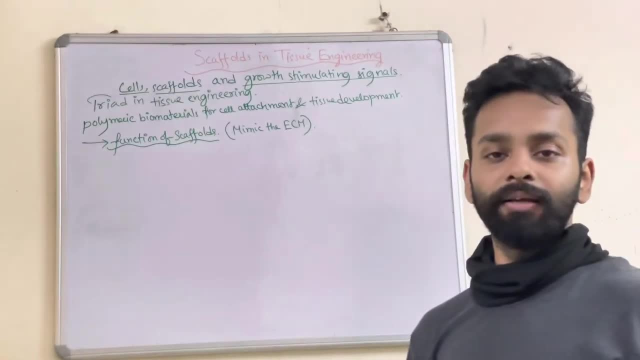 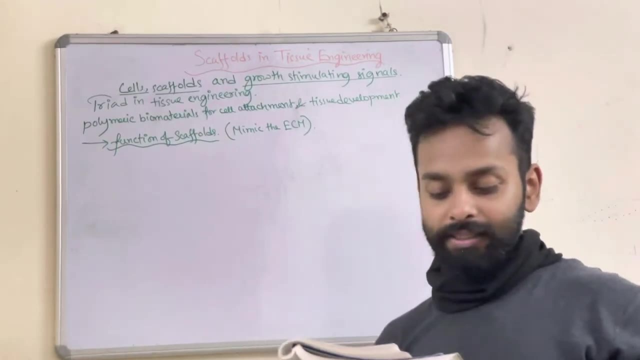 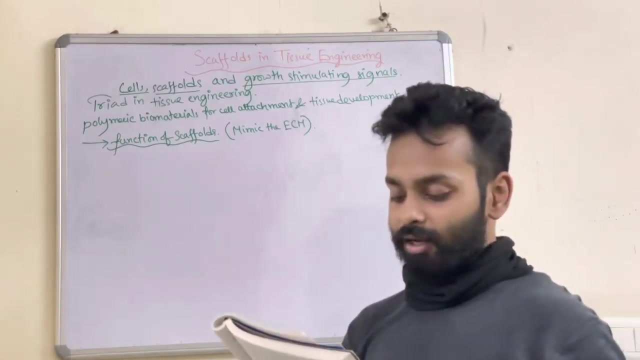 scaffold. A scaffold is basically a 3D material which is used to provide structural support for cells attachment and contact characteristics. So the scaffold is a 3D material in which it is used to provide structural support for cells attachment and contact and subsequent tissue development. So a 3D material can be made up of polymeric biomaterials. 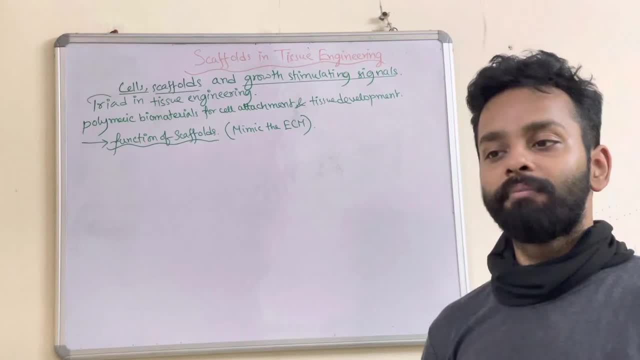 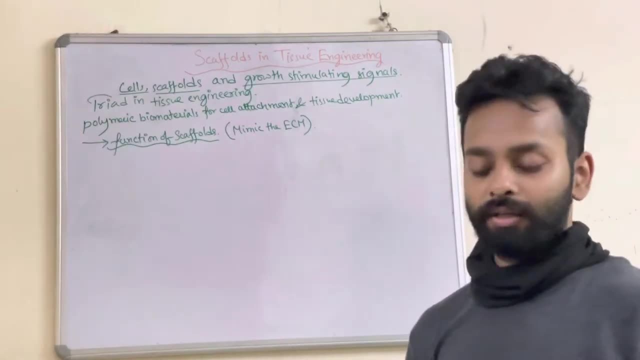 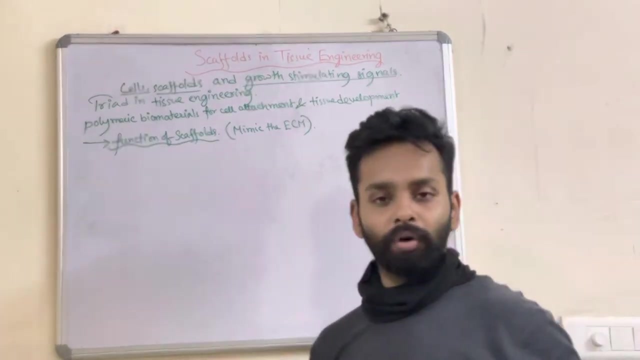 which can be used as a supporting framework or a supporting material to provide structural support to the cells for cellular and tissue development and differentiation. So functions of the scaffold. So what are the main functions of the scaffold? So most cells in our body are anchorage dependent. So the cells need a specific substrate or 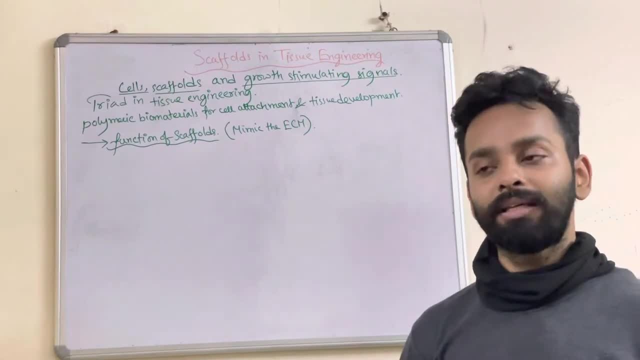 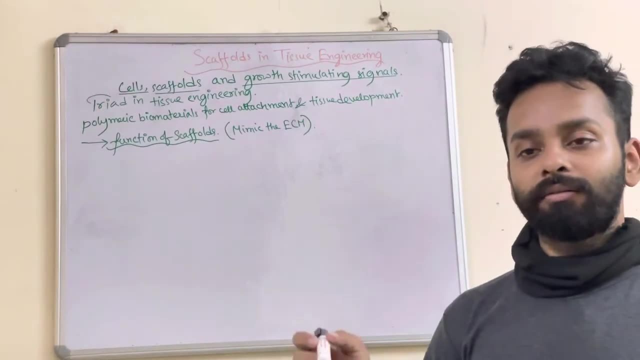 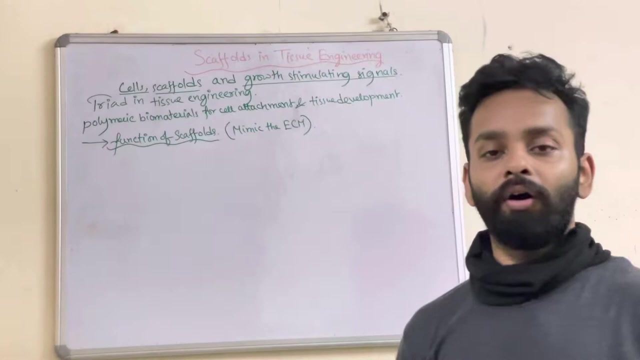 a substrate to grow and attach to it. So once they are attaching to the substrate, Theythrough different molecular interactions they arethey get spreaded and assume a specific morphology, and these types of cells are known as adherent cells, or and these cells. 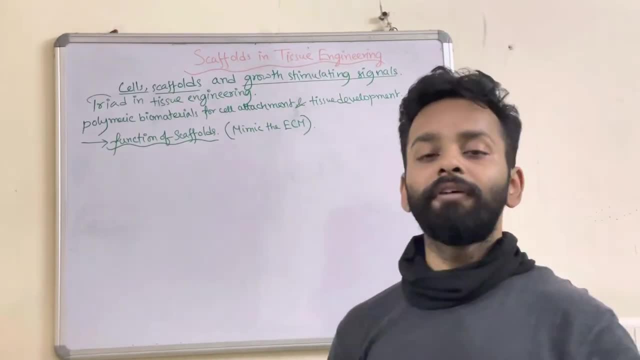 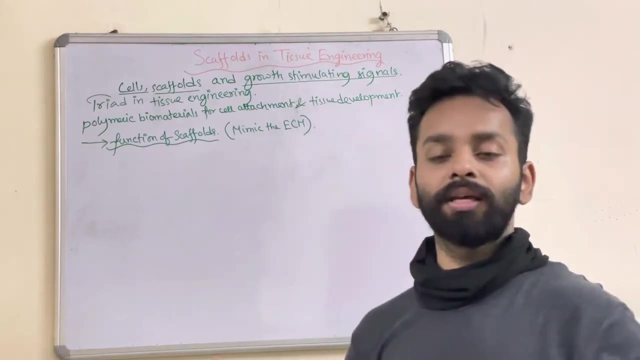 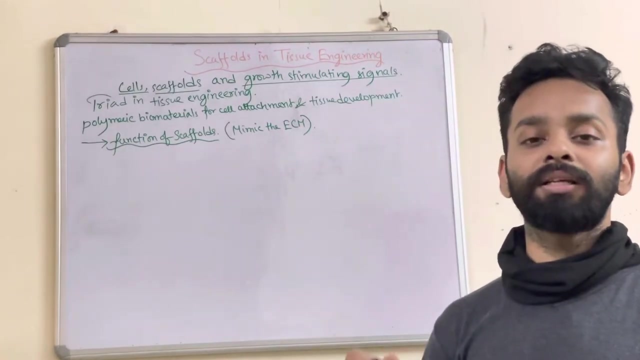 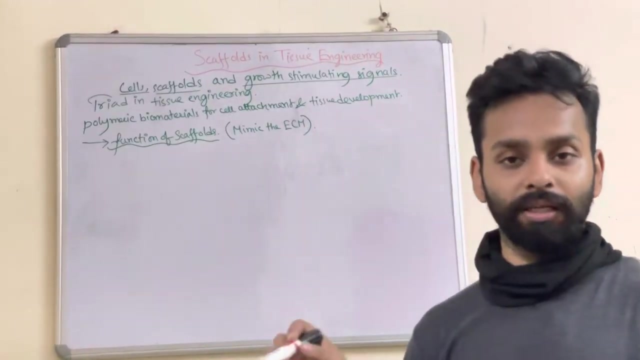 usually grow in a monolayer, But in in vivo conditions, these cells are scaffolds, enable these cells to. since these scaffolds are porous structures, these scaffolds enable the cells to migrate through their pores and therefore allow a three-dimensional structure or a space for the growth of the cells. Now, when cells are growing in a three-dimensional space, 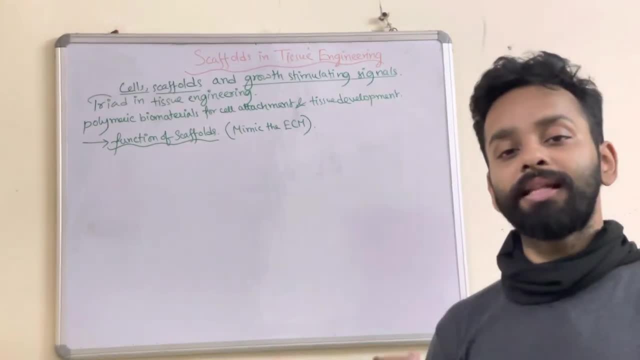 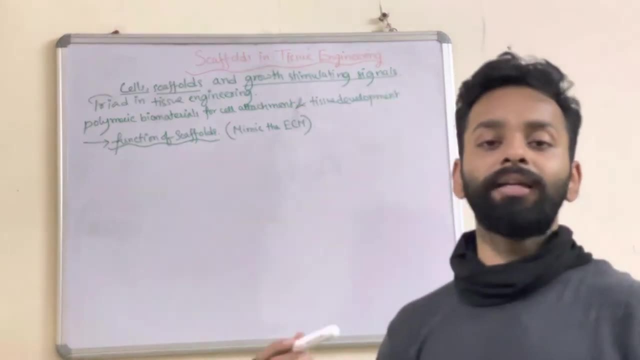 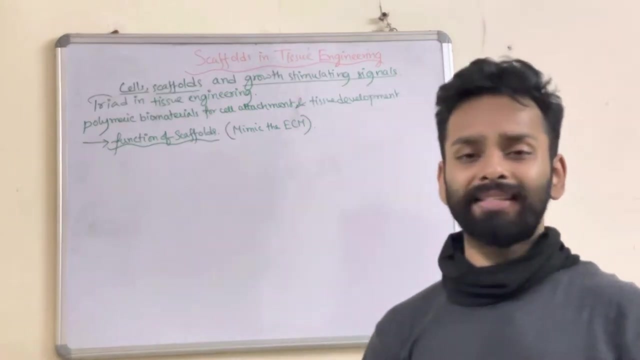 rather than in a monolayer, then these cells start behaving together like a tissue. So these cells start assuming or getting a tissue like morphology and also assuming their specific functions, such as secretion, signaling and many other associated functions which are usually found in tissues. 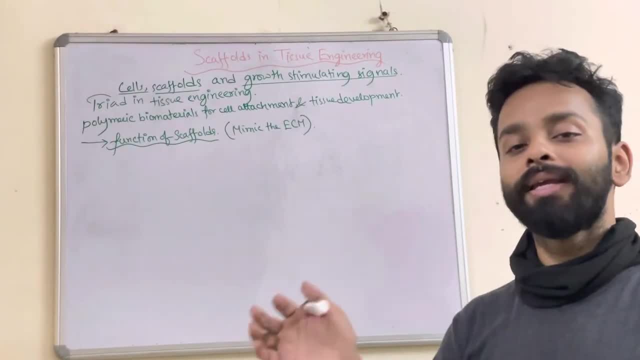 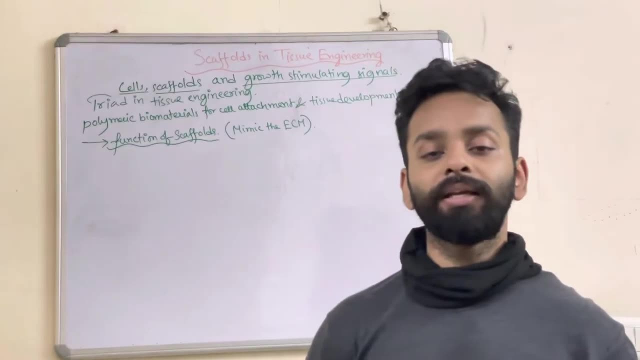 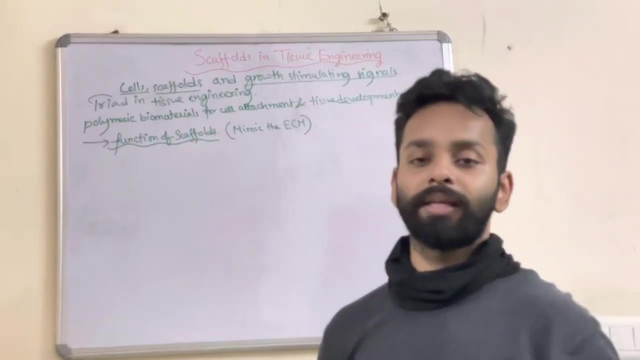 So cells will start assuming those functions once they are allowed to grow in a three-dimensional space. So the basic role of a scaffold. why a scaffold is used? so that it can mimic the physiology and the function of activity. So the scaffold is used to mimic the conditions of extracellular matrix, where different types of cells 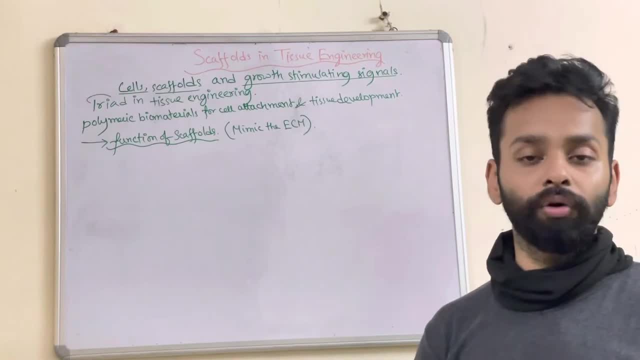 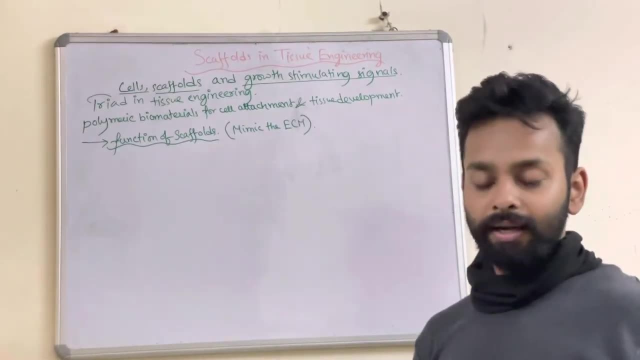 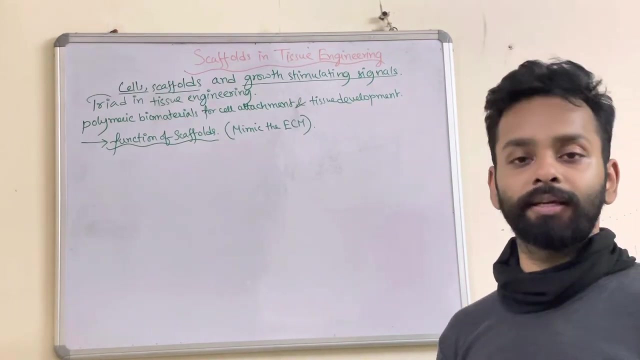 adherent cells grow in in vivo conditions. So most of these cells which are anchorage dependent and they reside in this solid network or solid meshwork of proteins which is known as the extracellular matrix. So the function of a scaffold is to mimic the conditions of extracellular matrix. 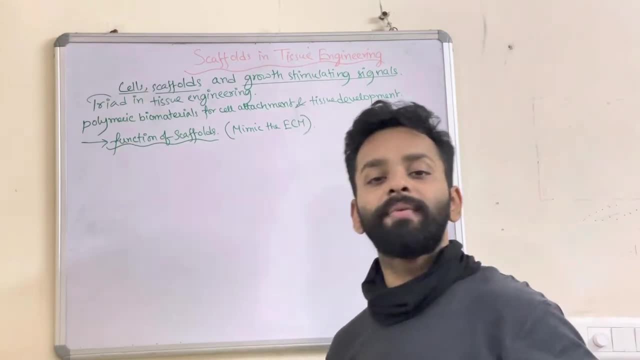 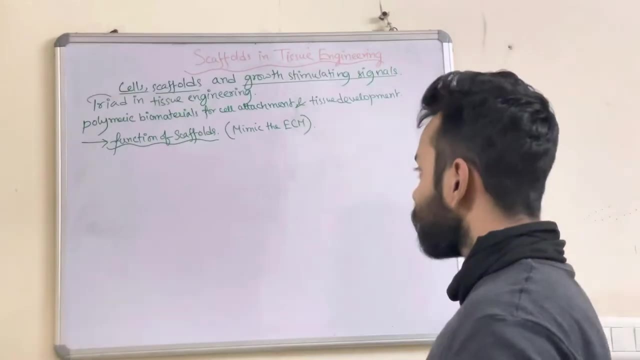 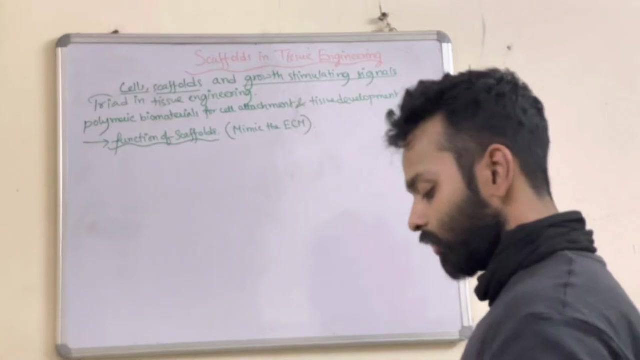 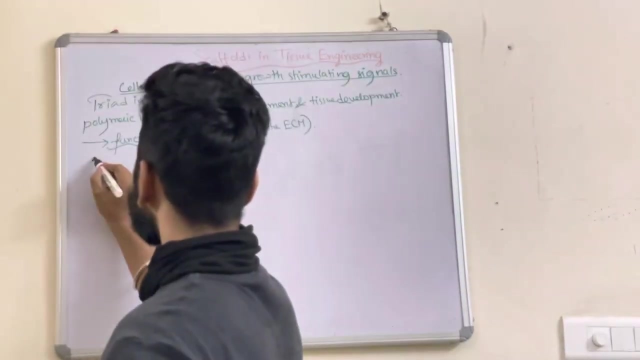 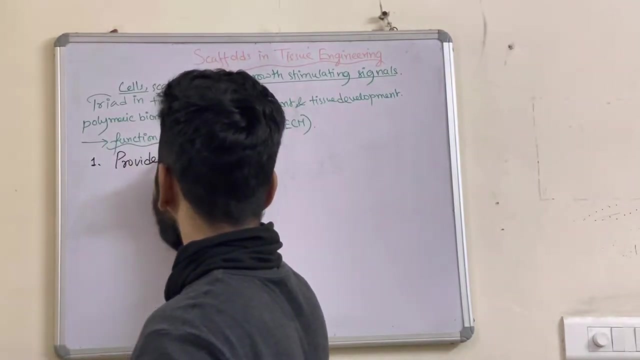 and thereby provide a three-dimensional growth space For the cells to grow and assume tissue-like function. So if we point out the different functions of a scaffold, so what we are essentially looking at include. So the first function, or the first important function of a scaffold is that it provides a structural framework. 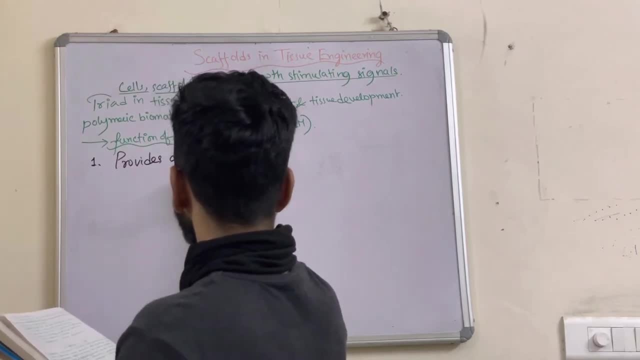 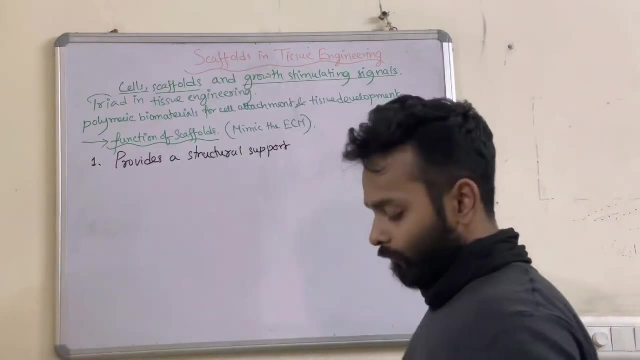 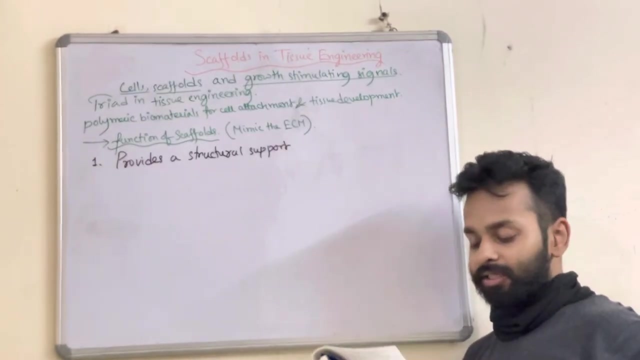 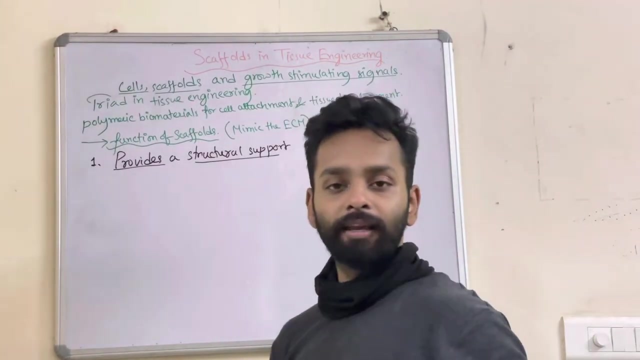 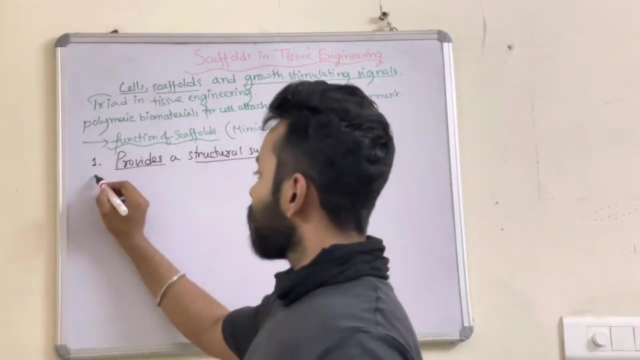 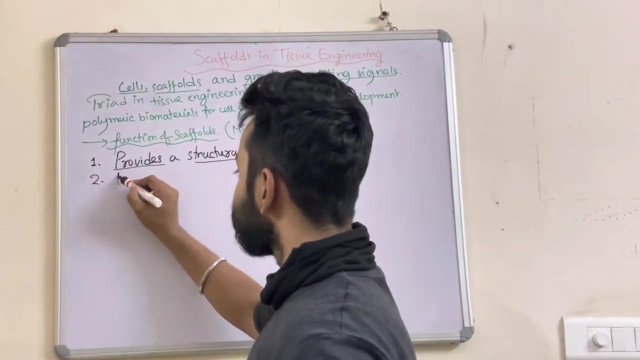 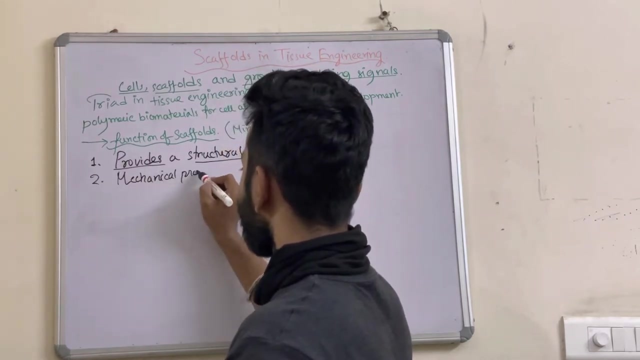 It provides a structural support for exogenously applied cells to attach, grow, migrate and differentiate in vitro and in vivo. So it provides a structural support for favoring cellular growth, differentiation and migration, both in vitro and in vivo. The second important function would be to contribute to the mechanical properties. 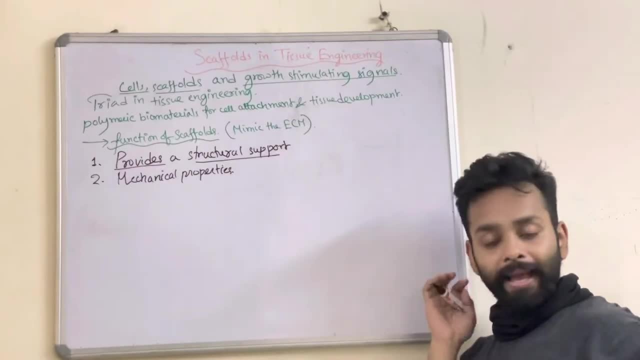 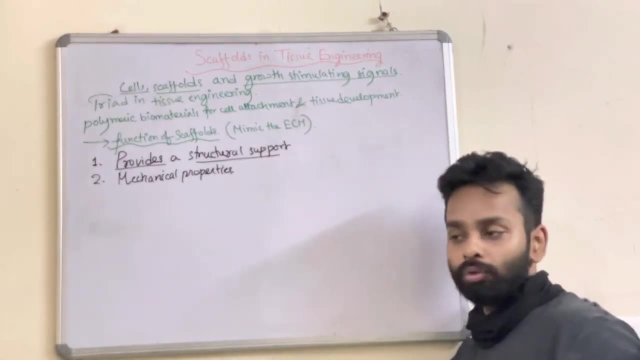 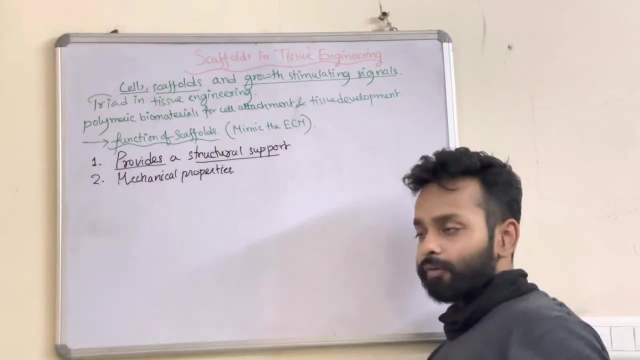 That is, scaffolds, will mimic the mechanical properties of the tissue in which it is being applied to, or the tissue which it is actually trying to mimic. So the mechanical properties of the tissues it will be trying to be similar to it and it will provide shape and mechanical stability to the tissue defect where it is trying to. 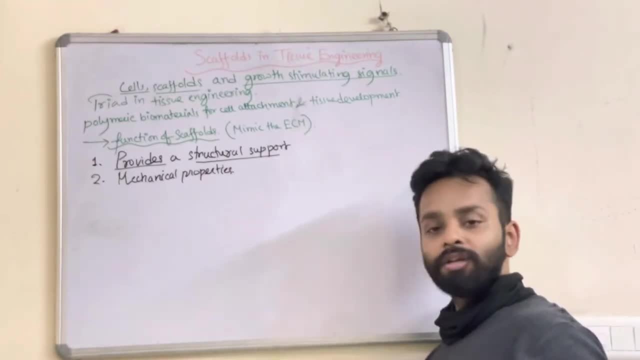 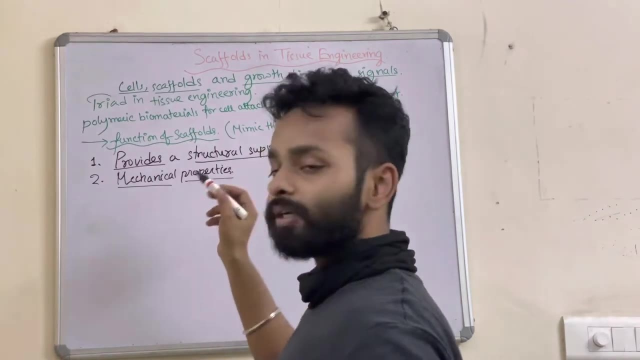 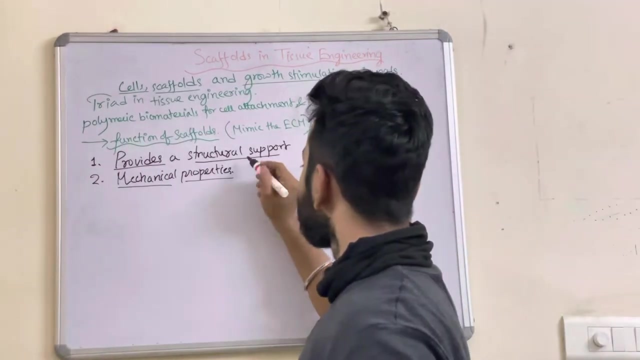 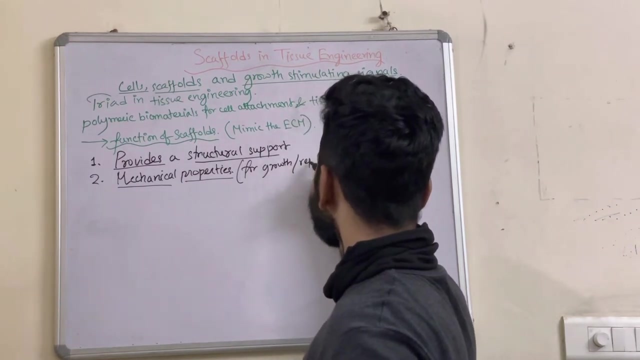 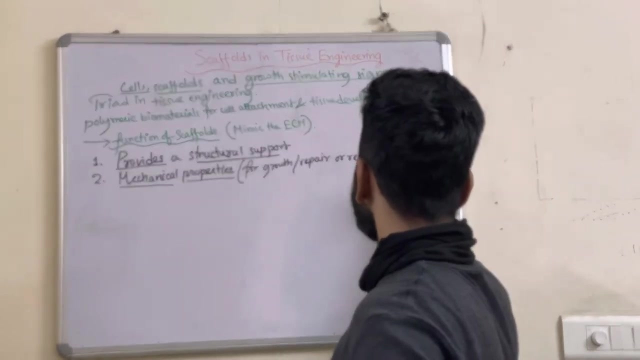 be used for and also give rigidity and stiffness to the engineered tissue. So this, the second point, would be to mimic the mechanical properties of the tissue, which is tissue system which is being used For repair or replacement, for growth, repair or replacement. 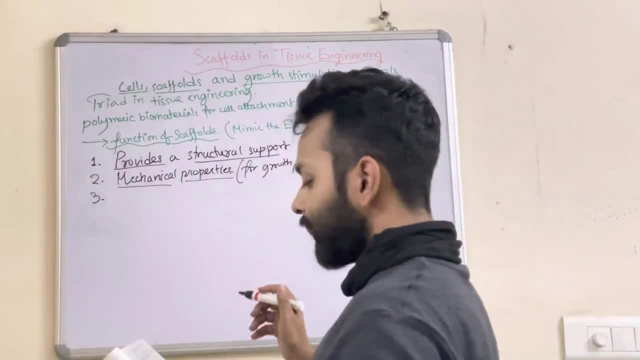 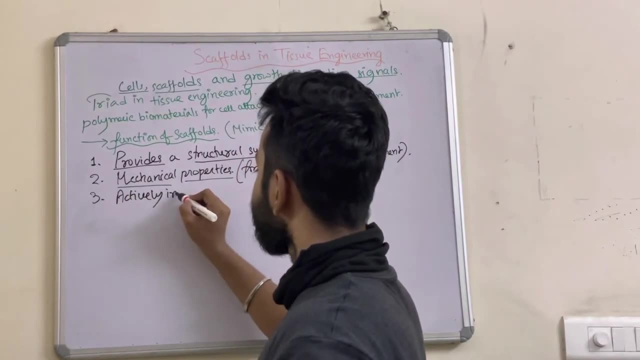 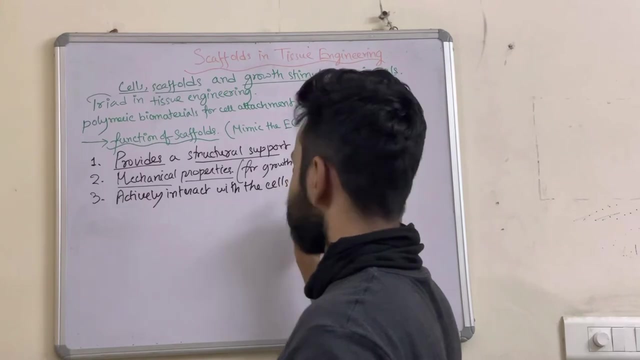 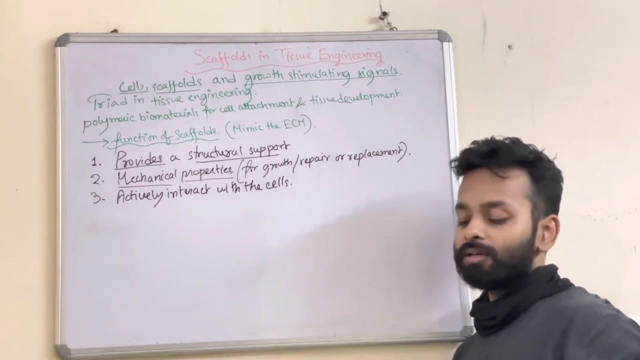 The third function would be to interact with the cells actively. So to actively interact with the cells. So to actively interact with the cells, So to actively interact with the cells And to facilitate activities such as proliferation and differentiation, which are very important characteristics of tissues. 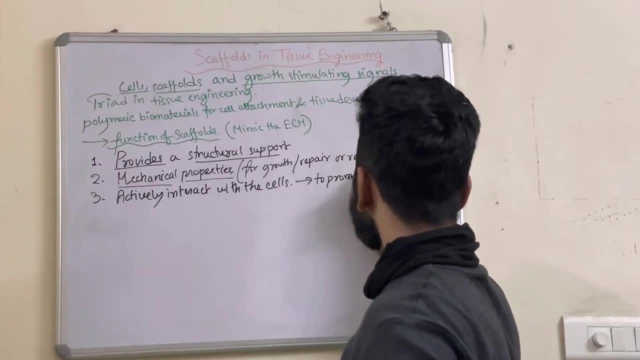 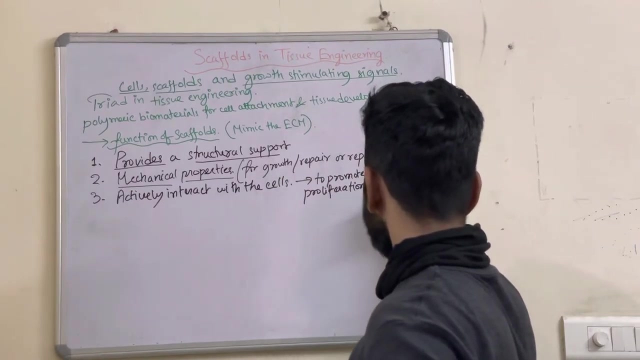 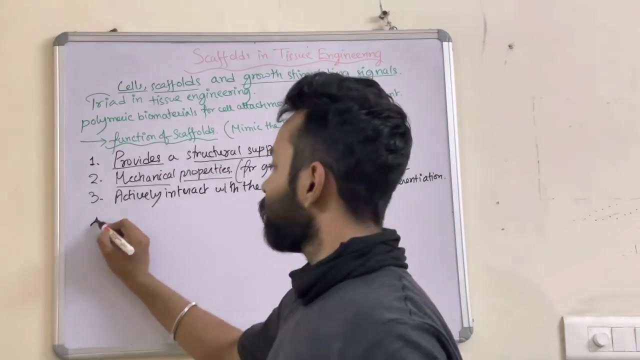 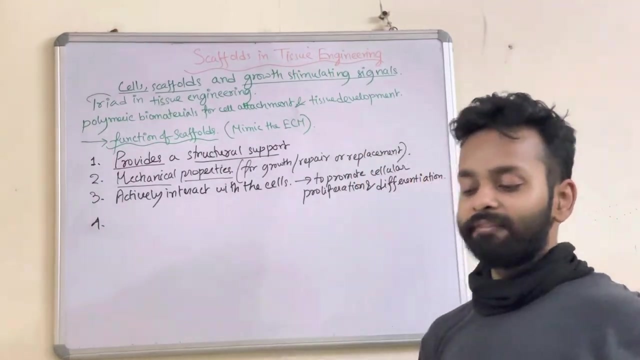 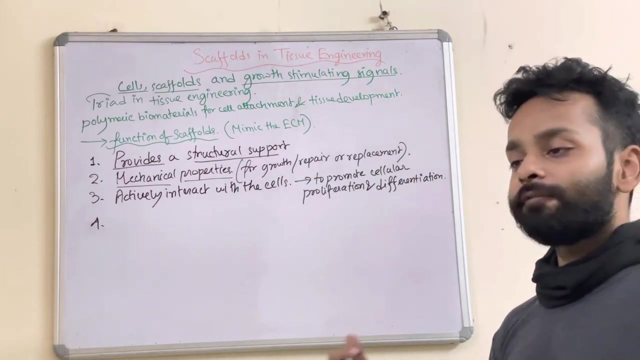 So to promote cellular growth, proliferation and differentiation. The fourth function of scaffolds would be that scaffolds might be used as delivery vehicles and reservoirs for externally applied growth stimulating factors. So these scaffolds might be prepared or might be added with growth stimulating factors. 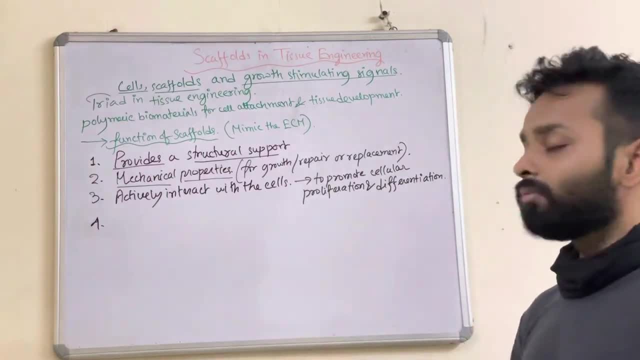 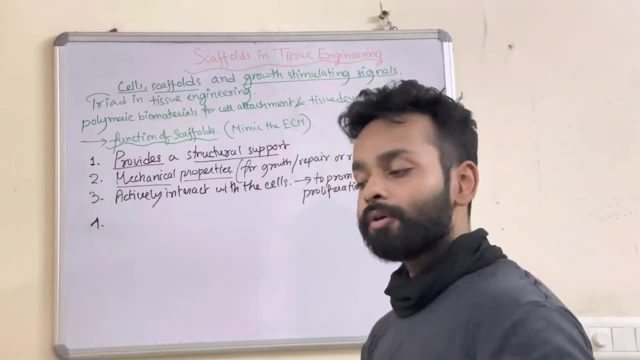 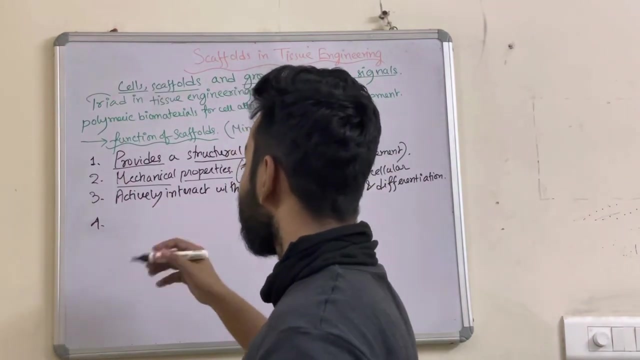 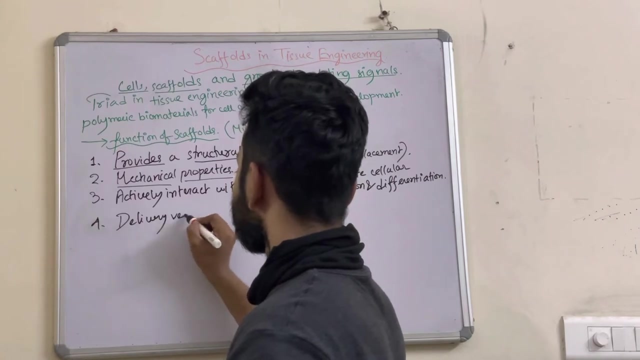 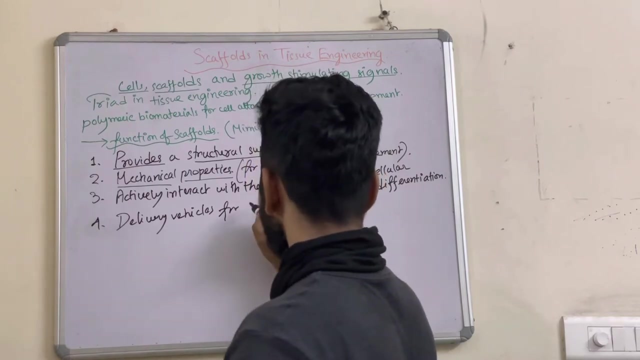 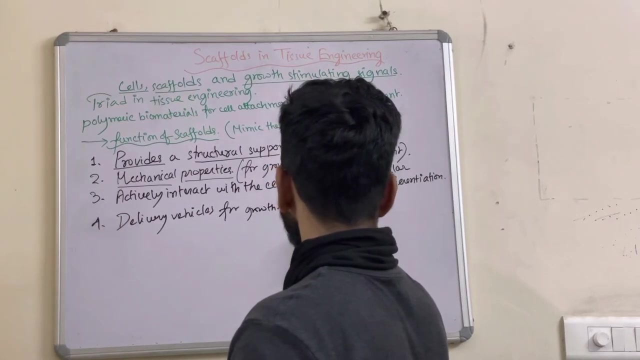 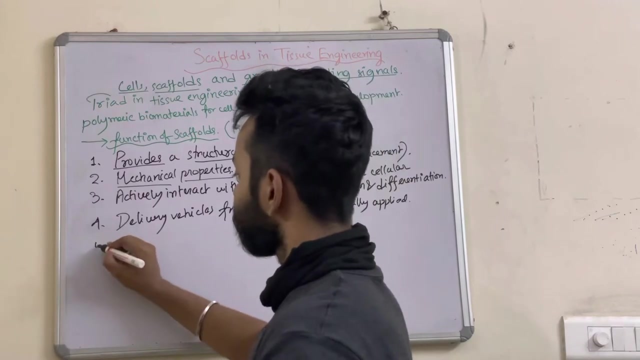 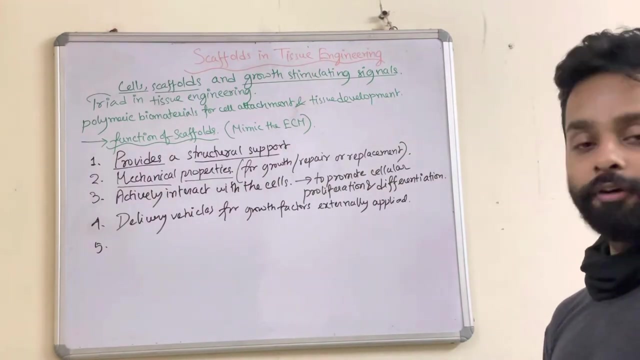 hormones or signalling molecules to enable these tissue differentiation, growth, development and proliferation and related dynamic behaviours of cells in tissues. So it will be acting as delivery or as delivery vehicles. Finally, another important function of scaffolds might be that it will provide a void volume. 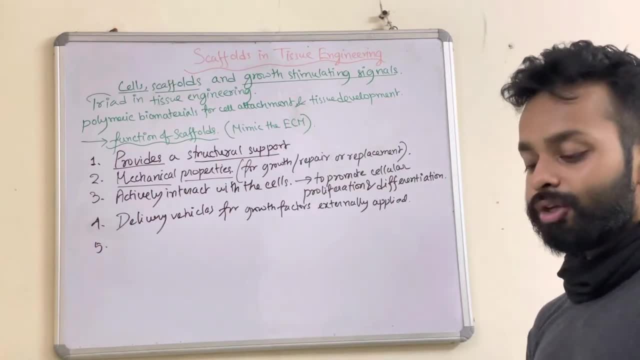 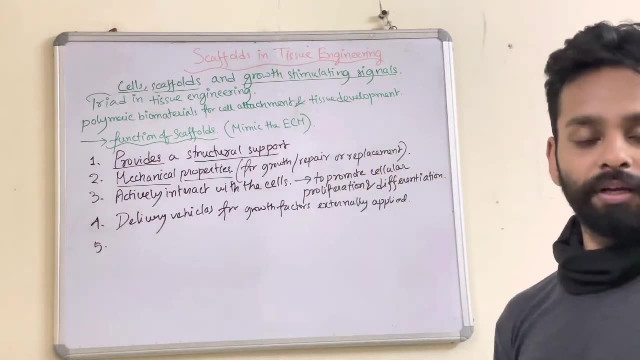 for enabling vascularisation and new tissue formation during the process of tissue remodelling. So some of the dynamic behaviours of tissues are influenced by these scaffold materials, once they can be fabricated with externally applied growth factors, hormones etc. to mimic the dynamic behaviours of tissues. 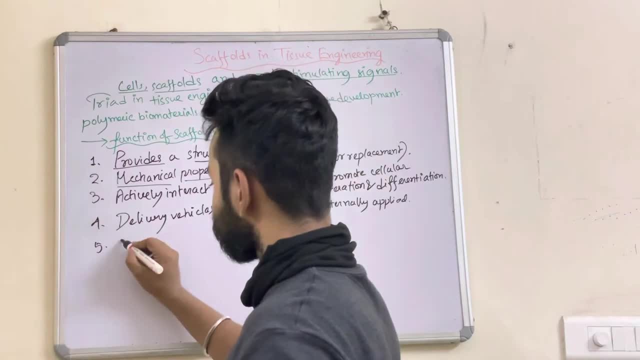 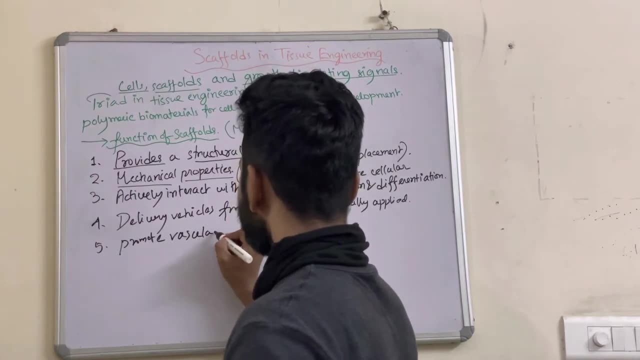 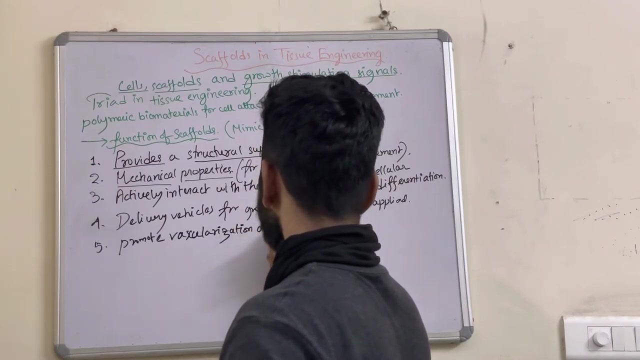 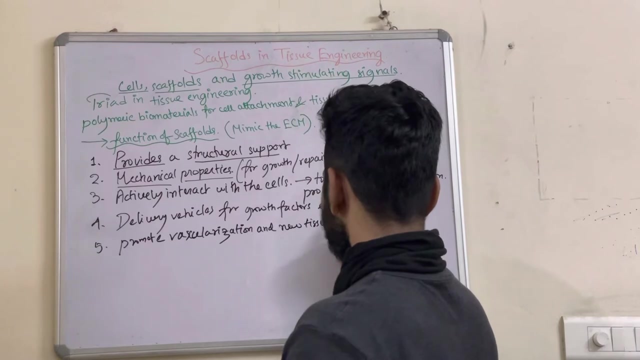 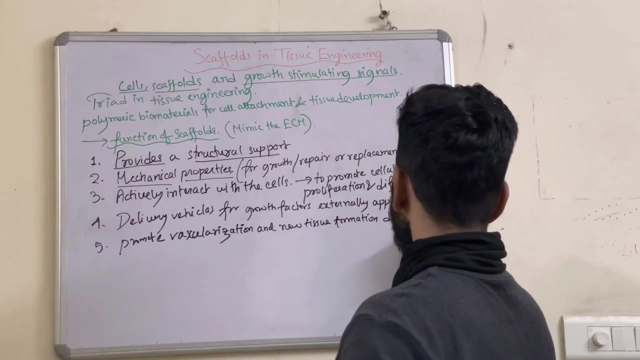 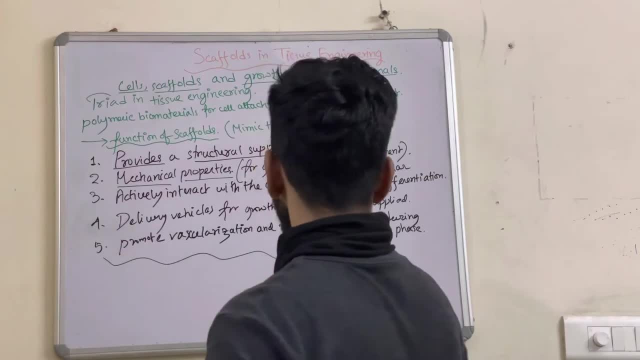 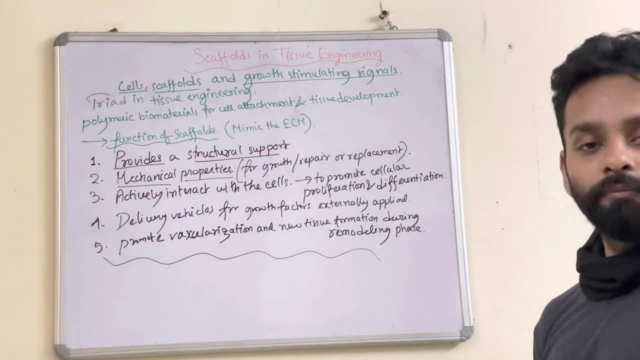 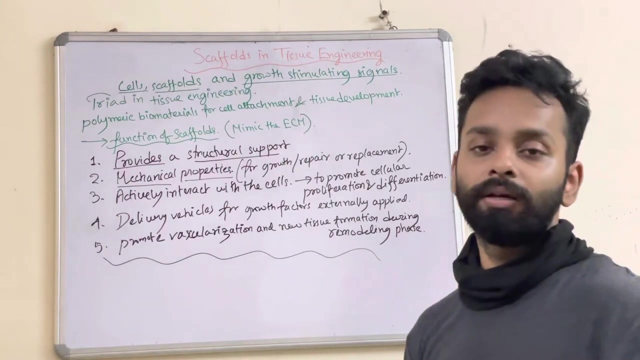 Vascularisation. So these were some of the important functions of the scaffold. So structure support, mechanical frameworks, stability, delivery agents and voting different dynamic behaviours of cells which make up the tissue Include or summarize some of the mitad functions of scaffold and why they are used in tissue. 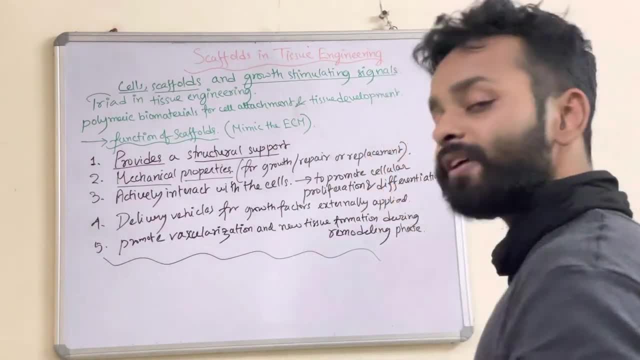 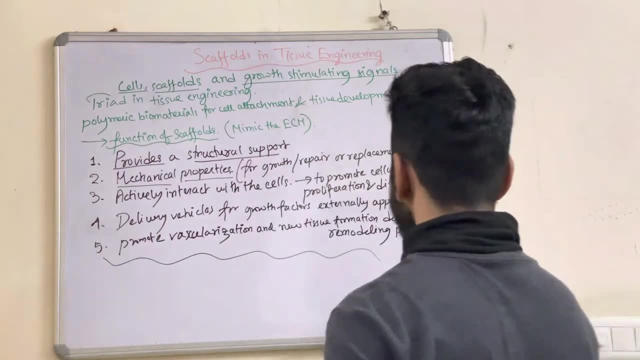 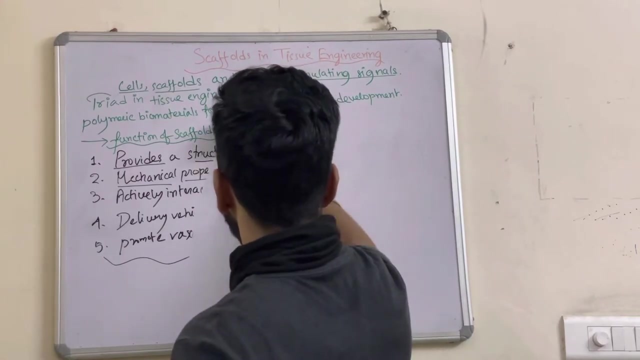 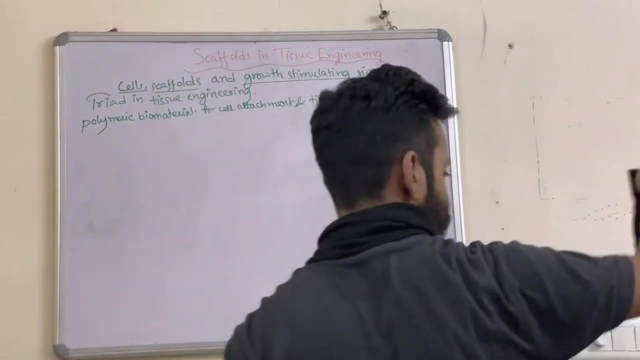 engineering. So now we will look at some of the compensations. We will look a some of the processes in which scaffolds are implemented physically in tissue, some features or characteristics of such scaffolds. So let me erase out some of this part. So 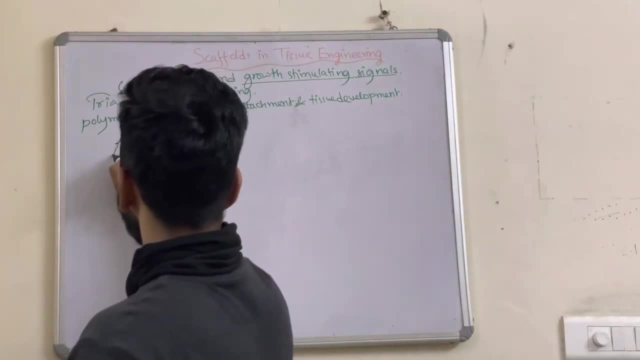 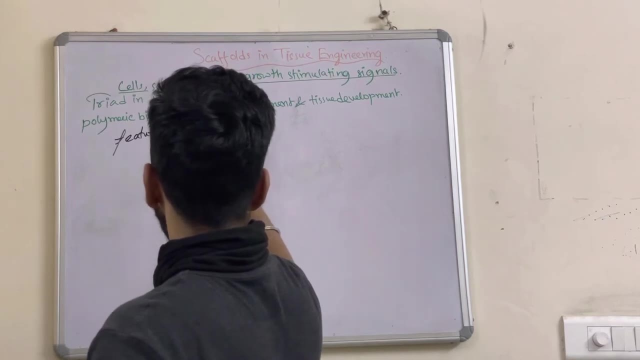 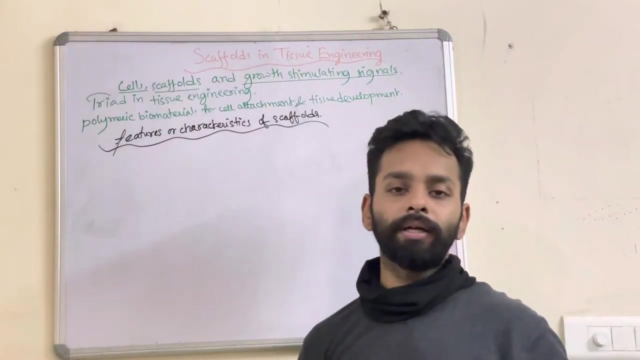 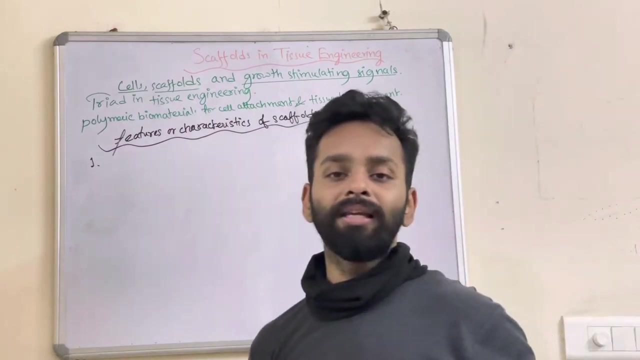 this will be looking now at some features or characteristics of scaffolds. So one of the very important characteristics of scaffolds will be their structure. Their structure is will be a highly porous structure. So porosity is a very important, essential feature of scaffolds. 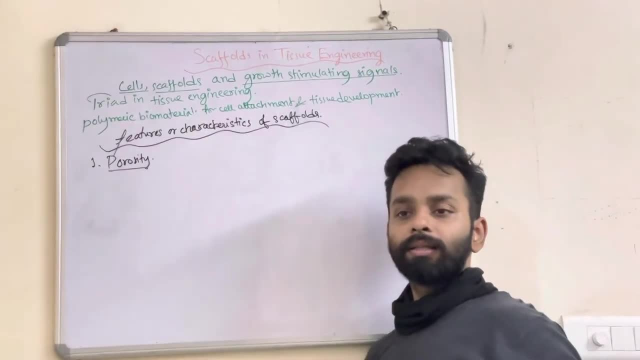 So porosity represents the percentage or the total amount of pores which are present in a given material. So why are pores important in scaffolds? So, as I mentioned before that scaffolds mimic a three-dimensional growth space or growth environment for cells, for 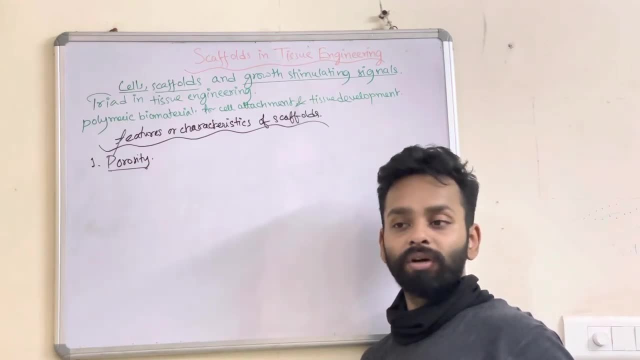 stimulating or for mimicking the tissue, like behavior, or tissue like morphology of the cells. So that is why this porosity, or the pore structure in the scaffold, is very essential, because to promote cellular migration and attachment inside the pores so that the cells can grow in a three-dimensional growth space or a growth environment. So that is why porosity 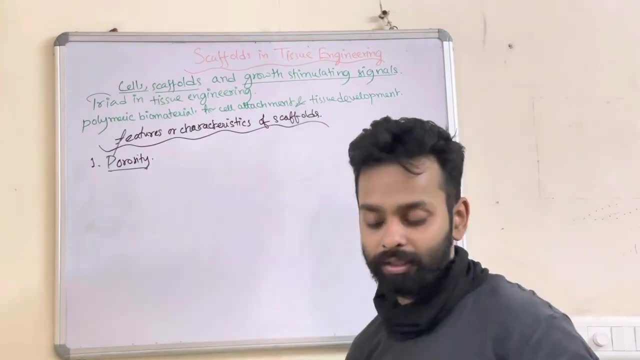 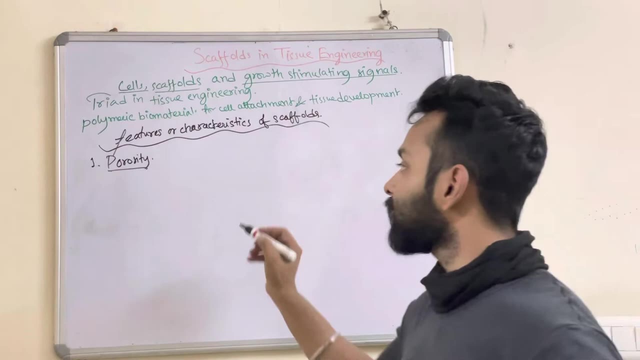 the total amount of pores in a given material or a given volume of a material, so it can be measured in different ways. so these scaffolds will have a porous structure and also the pores will be interconnected, so interconnectivity is also an essential criteria in porosity. 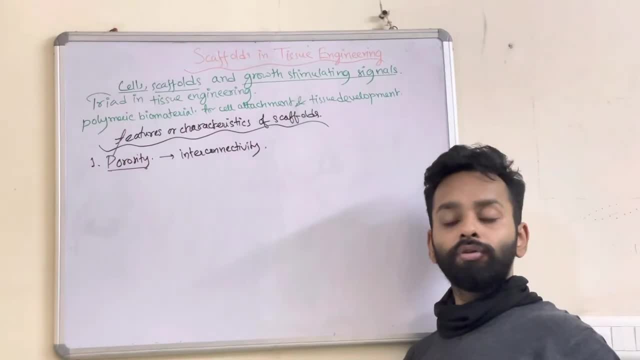 and these pores will be interconnected in order to uh, in order to uh, stimulate or mimic the cross-talking between the cells or interaction between the cells which will be growing inside the, the pores, inside the scaffold. so material exchange, signaling all these activities will be, will be 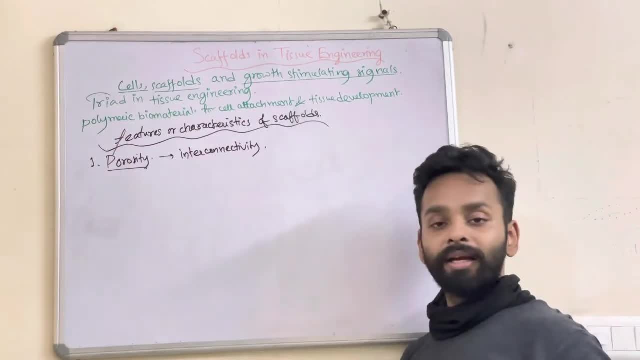 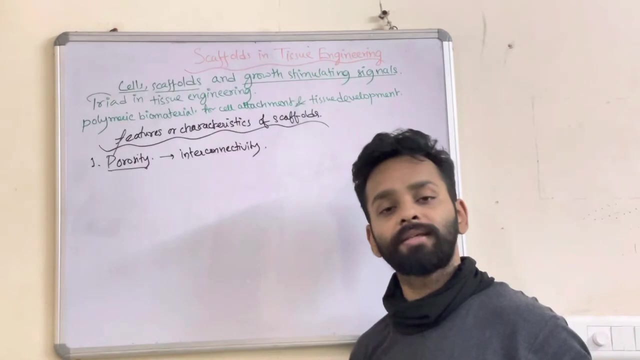 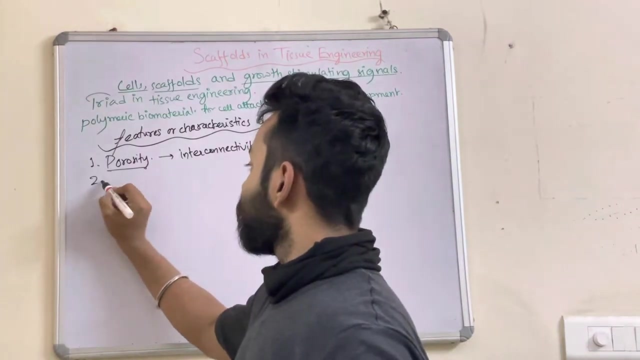 mimicked or will be facilitated by the interconnectivity between the different pores of these scaffolds and also based on this particular applications, these porosity can be controlled through different ways. so the different fabrication techniques of these scaffolds, which we will be discussing subsequently, the porosity can be altered or can be controlled. so a second feature of scaffolds would be: 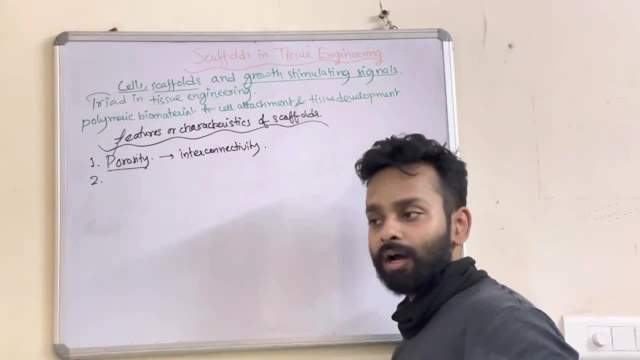 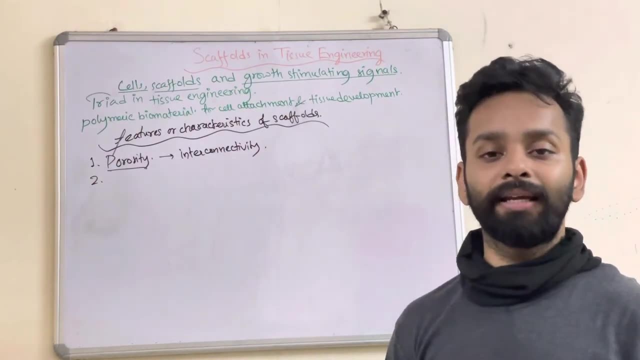 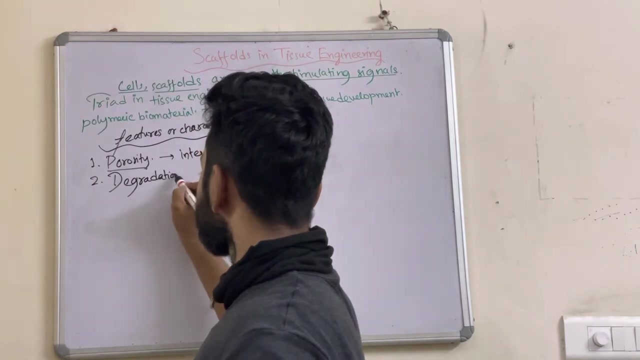 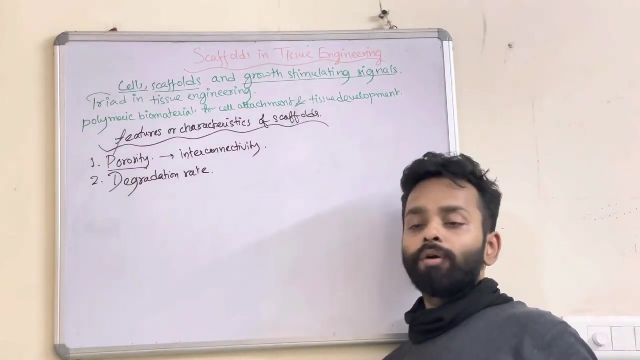 based on the type of application we are trying to develop for fabricating a specific type of a scaffold, these scaffolds should have a specific degradation rate. that is, since most of these scaffolds are used in viable systems for promoting wound repair, such as i have given an example previously, that is, for a third degree burn, we can create a scaffold to 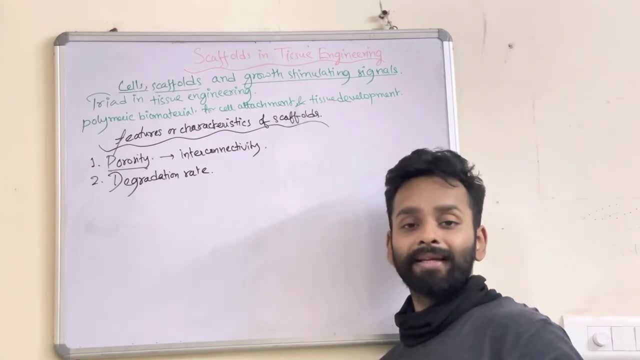 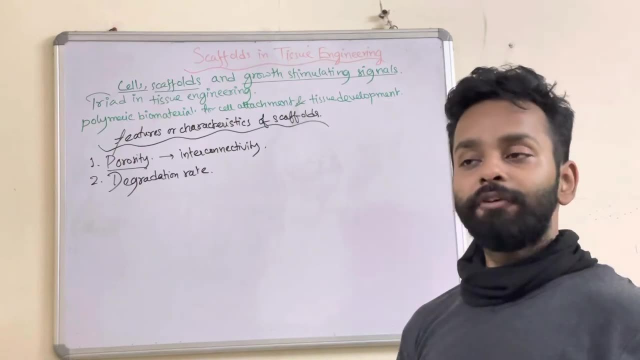 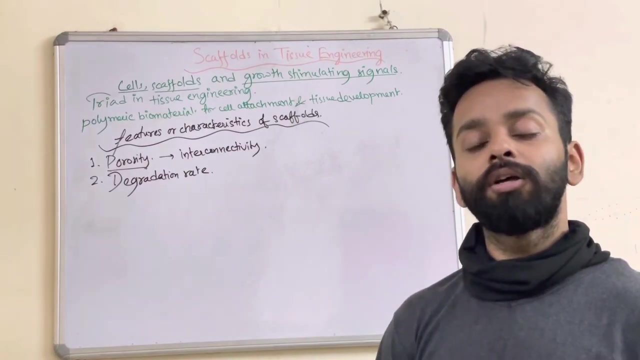 promote skin repair, or a scaffold to act as a skin regeneration template for treating patients with third degree burns. so in such cases, if we are implanting the scaffold with fibroblast cells inside a patient's skin So that scaffold slowly needs to be degraded so that it can be replaced, 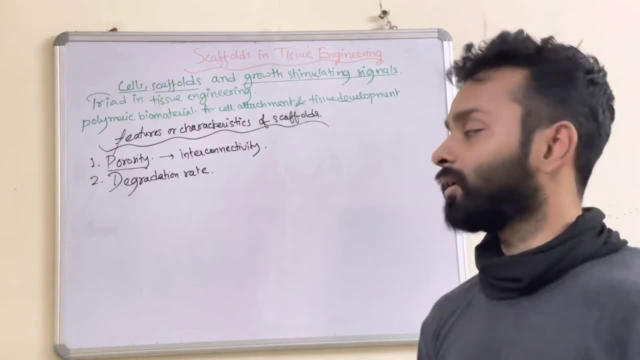 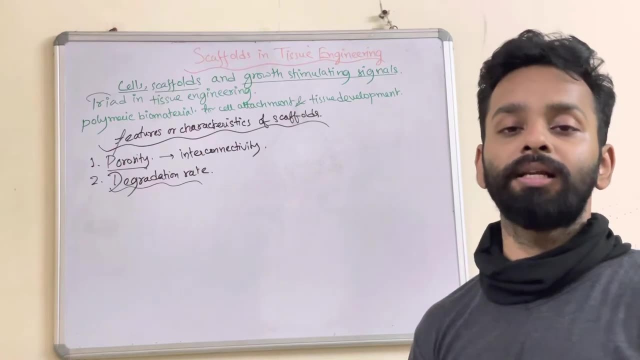 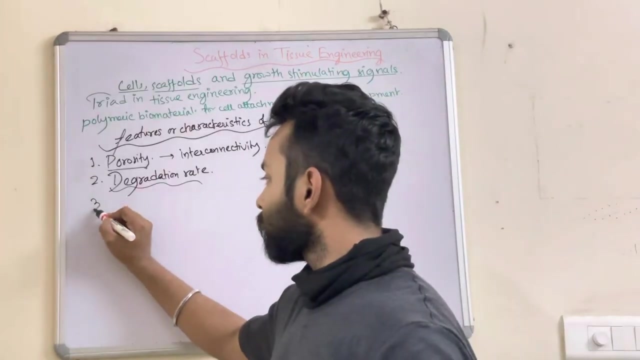 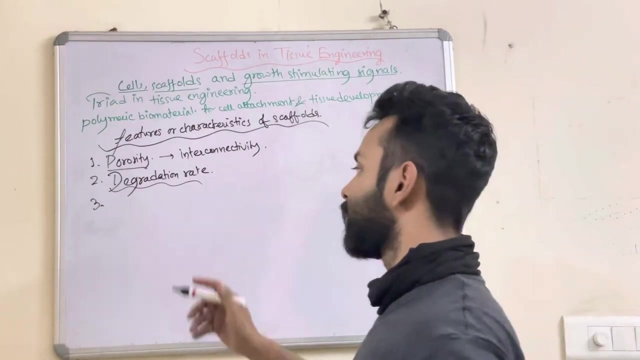 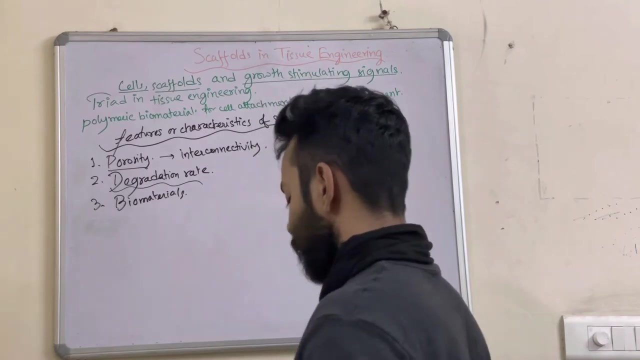 by normal skin, like tissue in the patient. So that is why a properly tuned or a properly controlled degradation rate is an essential consideration while fabricating any type of given scaffold based material. A third feature of this scaffold could be that these scaffolds can be fabricated with biomaterials, so that these biomaterials will have the sufficient 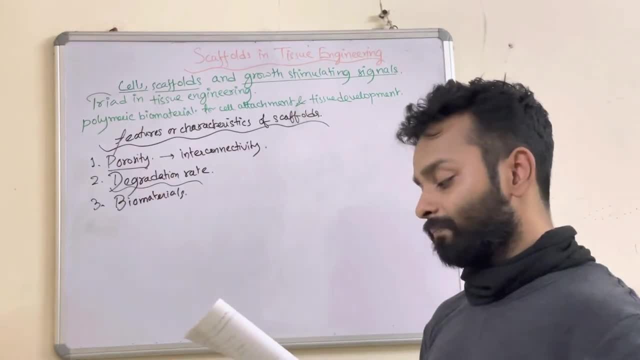 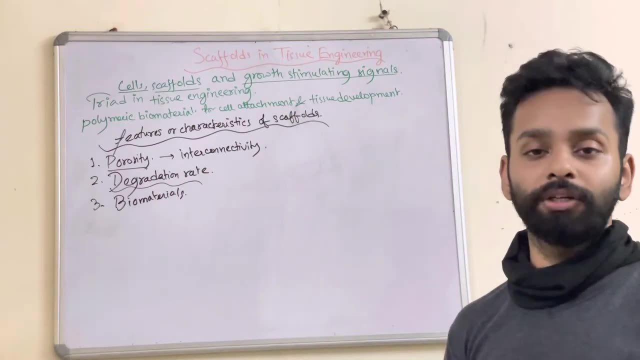 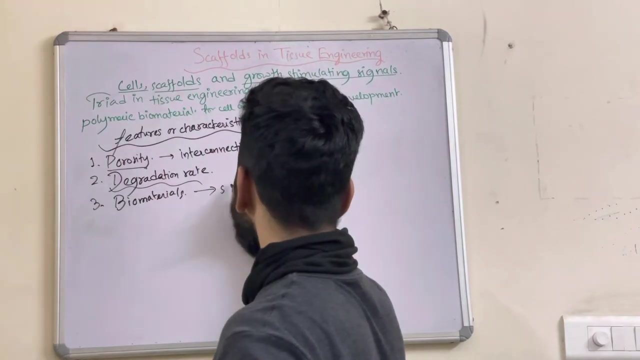 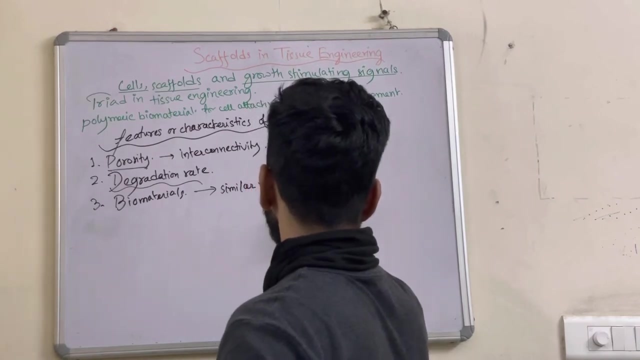 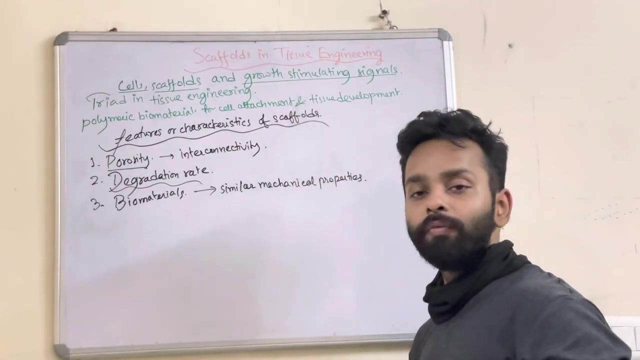 mechanical properties or desirable functions so that it can be actually used to mimic the type of tissue which we are trying to fabricate it for. So it should have the same or similar mechanical properties for the tissue in which it is desired to be used or where its application. 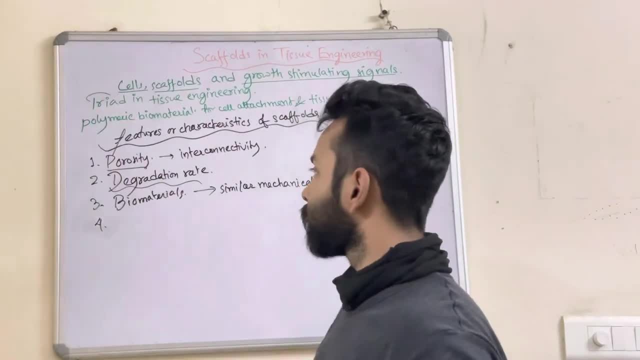 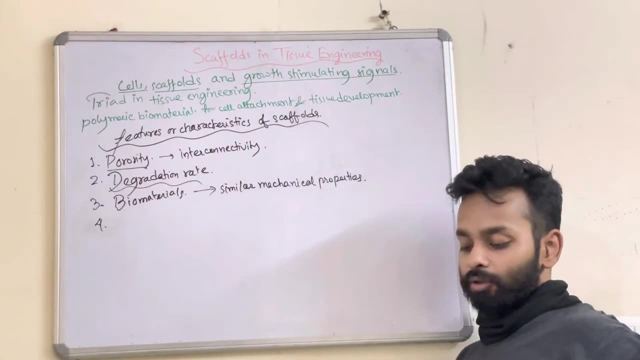 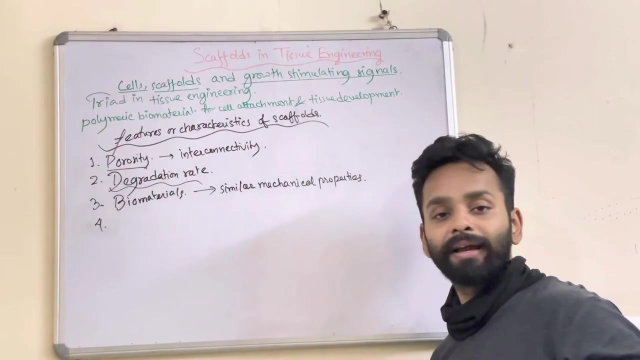 will lie. So the fourth characteristic would be biological cues, such as cell adhesion sites. physical cues, such as surface topography, should be present. So, as we just mentioned earlier, that these scaffolds might be used as used for adding a different growth factors or different hormones or different molecules to promote or the cellular 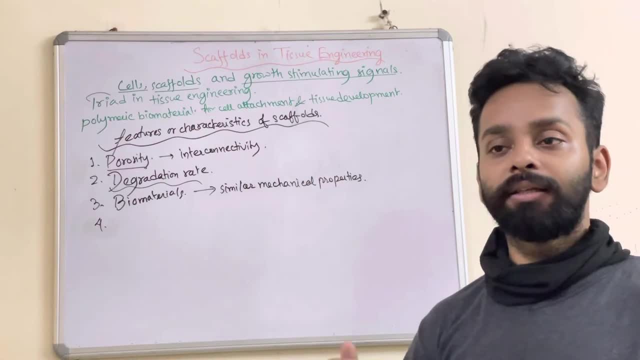 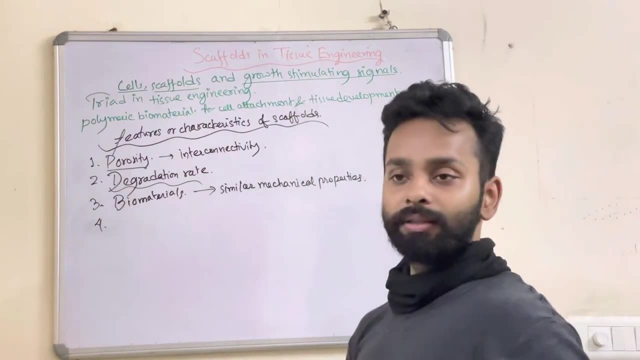 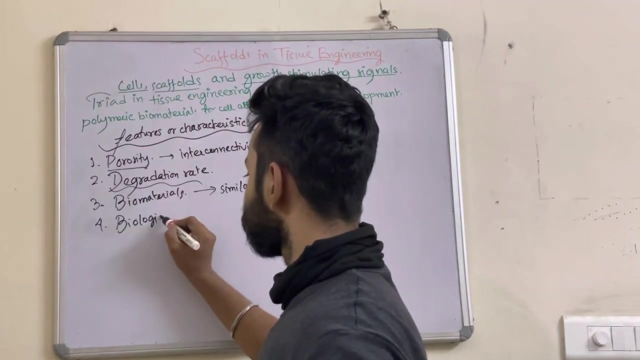 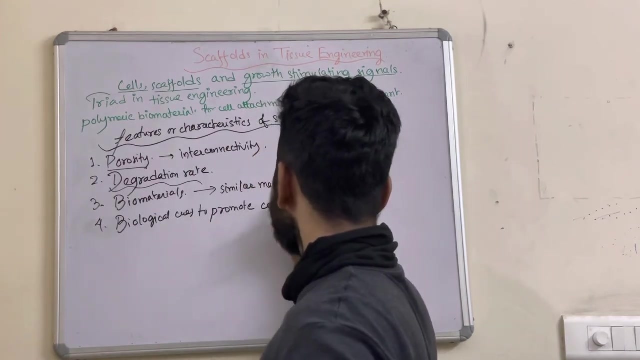 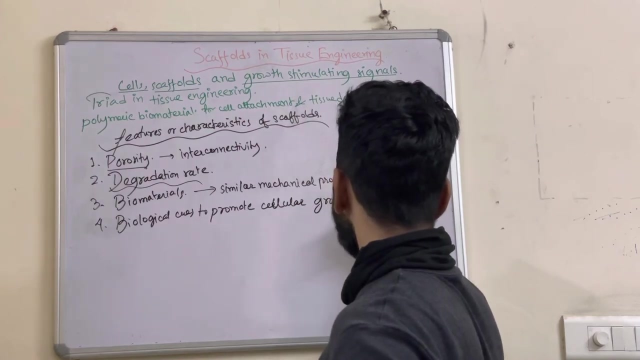 growth, migration and differentiation, thereby to mimic the different dynamic states of a tissue. So these scaffolds can be used. So these scaffolds can be added with, or can be provided with, different biological cues to promote cellular growth or proliferation, migration and differentiation. 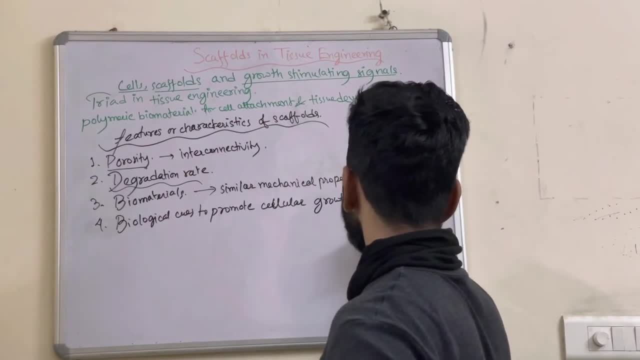 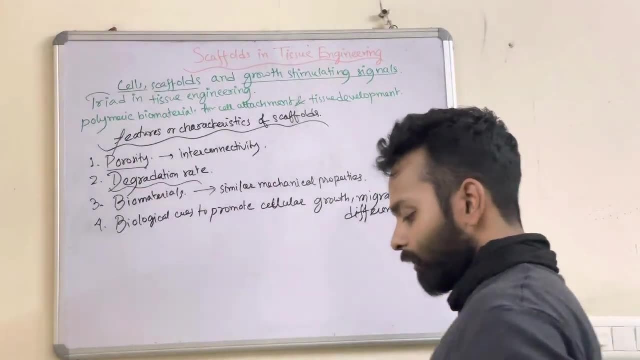 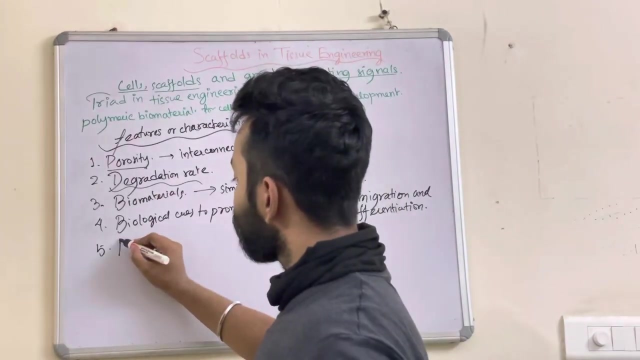 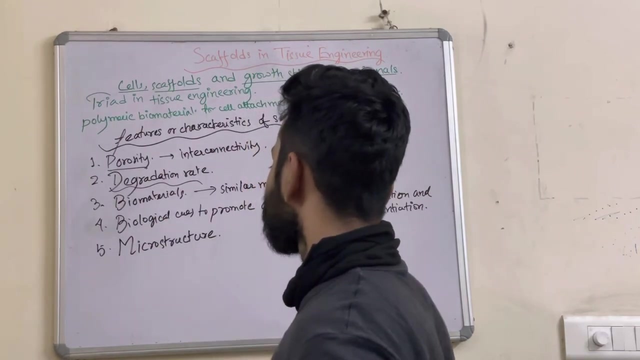 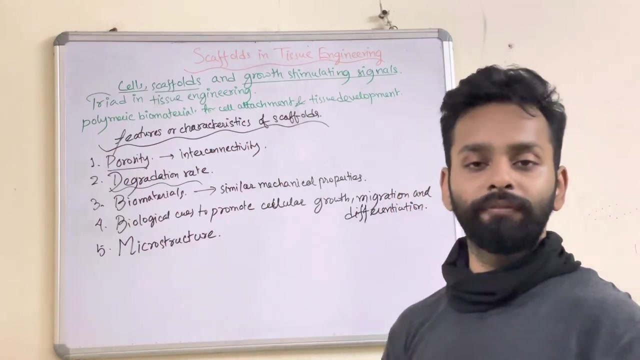 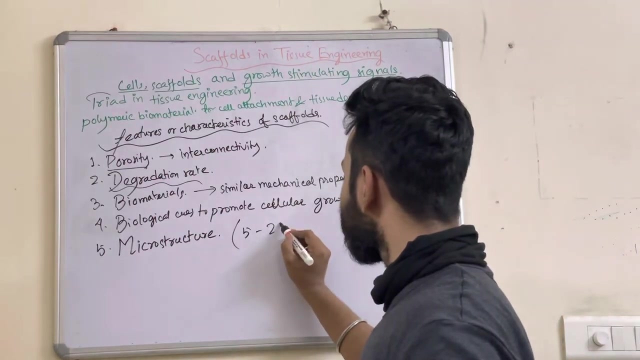 Thank you. The fifth feature of scaffolds would be that every scaffold should have a basic microstructure to promote the specific type of cells growth and proliferation which it is intended to promote. Okay, So eukaryotic cells can have a size range from 5 to may be 20 or may be 50. also micrometer. 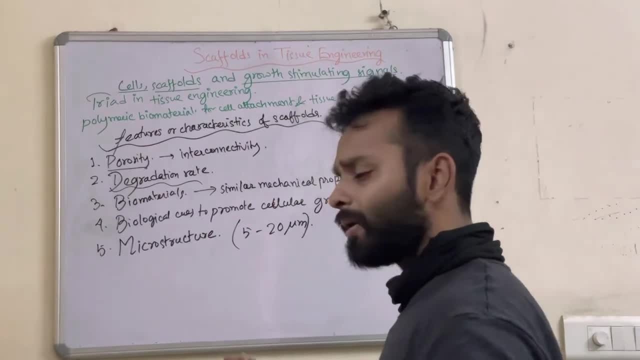 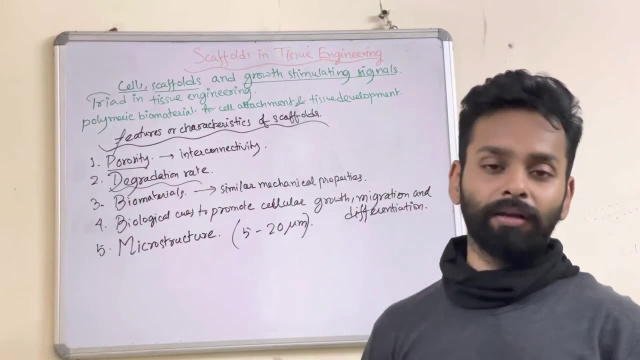 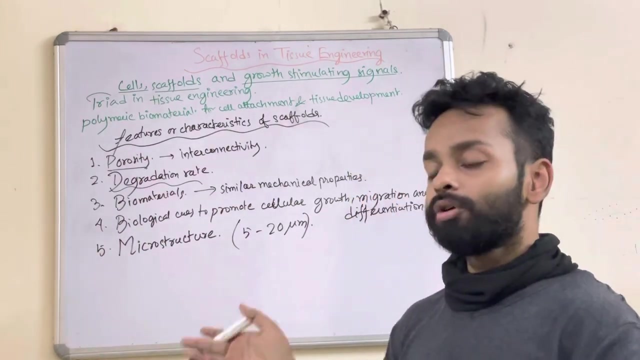 So, based on the type of cells which we are trying to fabricate, which we are trying to mimic using, or the tissue type which we are trying to mimic using a specific scaffold, So those pores should be in the range to allow those particular cells to migrate, grow. 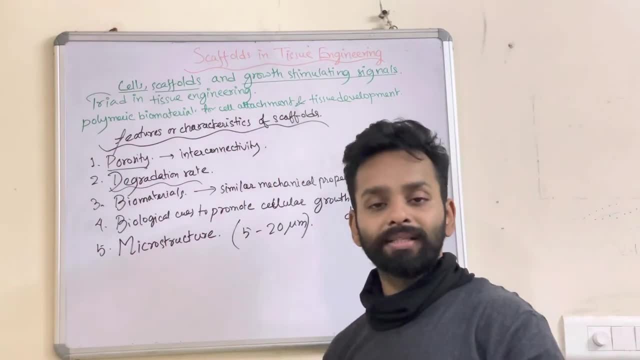 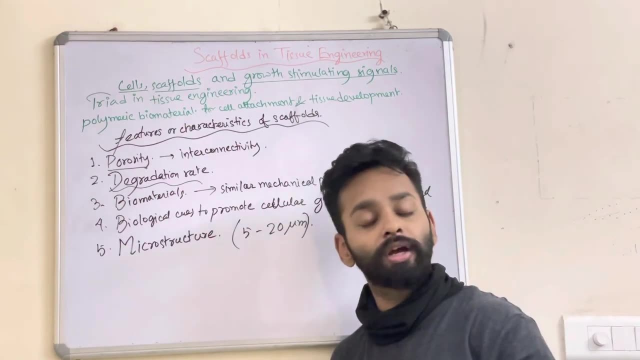 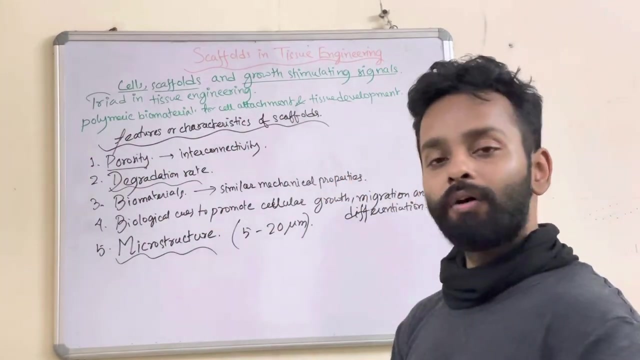 proliferate and differentiate. So if we are trying to make a skin regeneration template, we should enable, we should fabricate the scaffolds with pore sizes to enable the migration of fibroblasts right. So every scaffold should have a specific microstructure for its specific application. 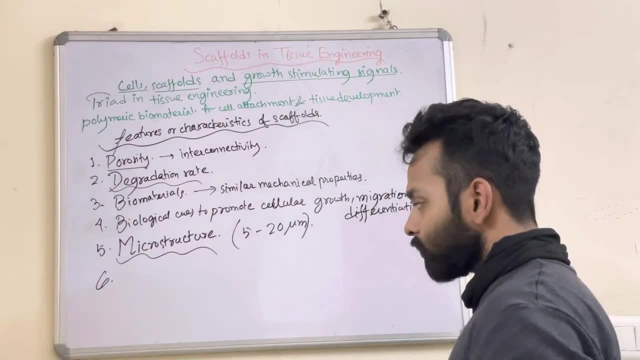 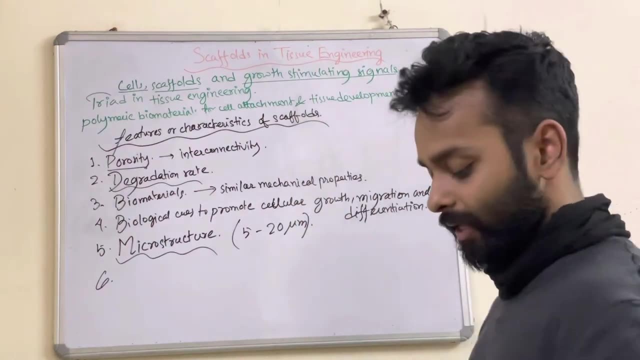 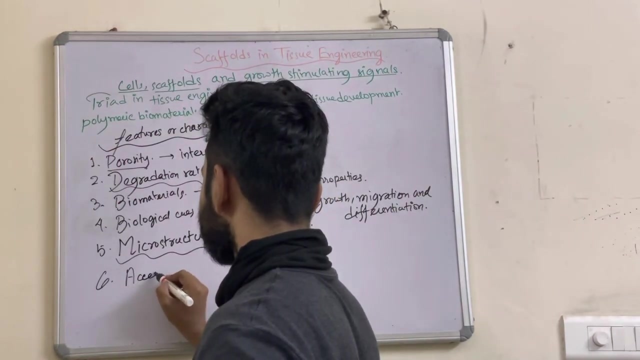 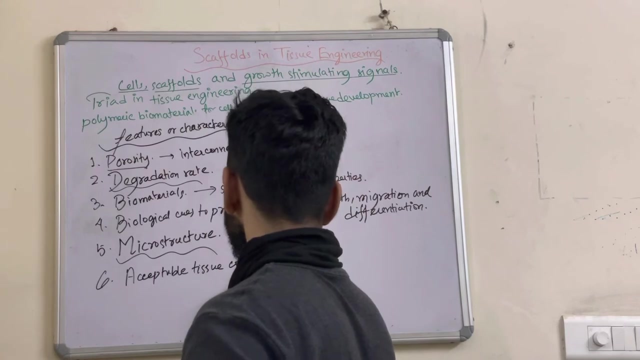 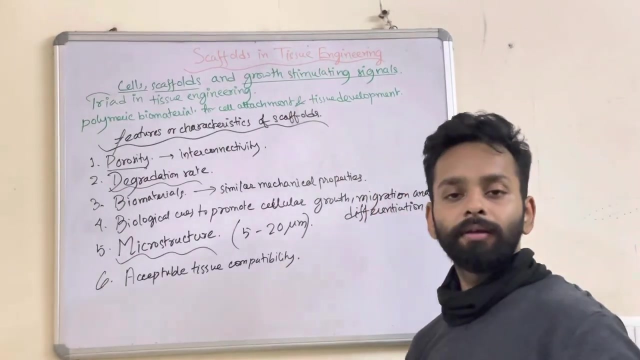 Finally, also one of the most, actually arguably the most important characteristic that any scaffold should have, is that it should have acceptable tissue compatibility, or biocompatibility. That is why, since we are trying to make a system which we will be using directly with,